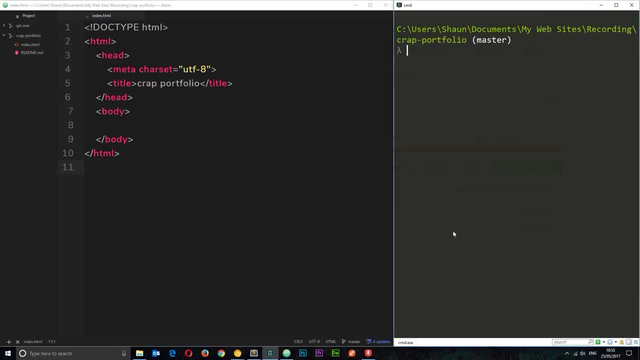 locally up to date with the remote repository, just in case any of the other developers has made any changes. So to do that, what I'm going to say is make sure I'm on master, first of all, the master branch, because that's what I want to. 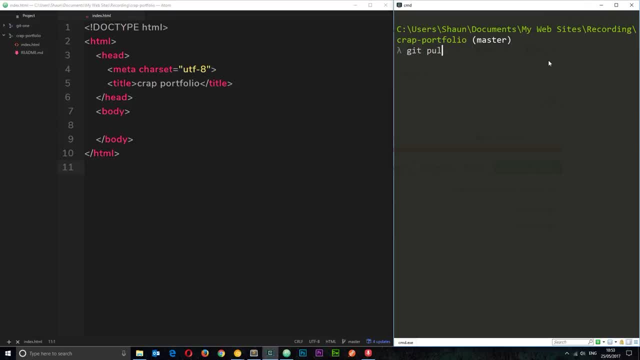 merge to. then what I'm going to do is I'm going to say git pull, and then I'll say the origin, because that's the alias we're pulling from, that's our remote repository, and then we're going to pull the master branch. So what a git pull does. 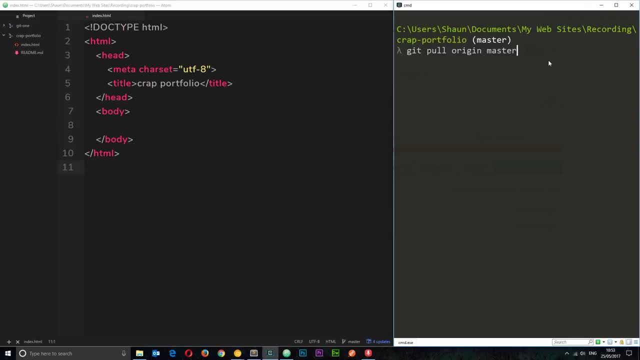 is. it fetches all of the files that I've got in this project and it's going to from the remote and then it merges it into our master branch, because that's what we've said right here, master right, and we're on the master branch, so it's. 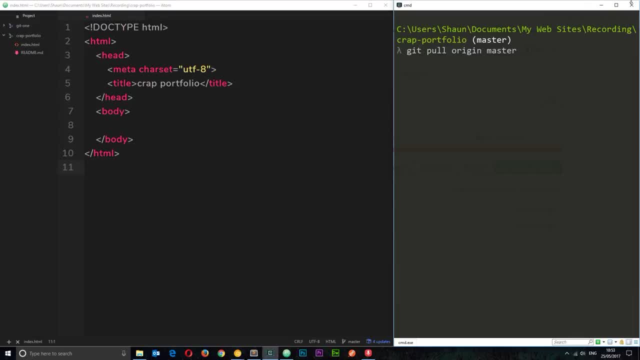 going to pull the master branch from the remote into the master branch onto our local and update all of the files. in this case no one's made any other changes and everything's already up to date. so that's fine. but I do that just in case there were changes that other people had made in the meantime. cool, so 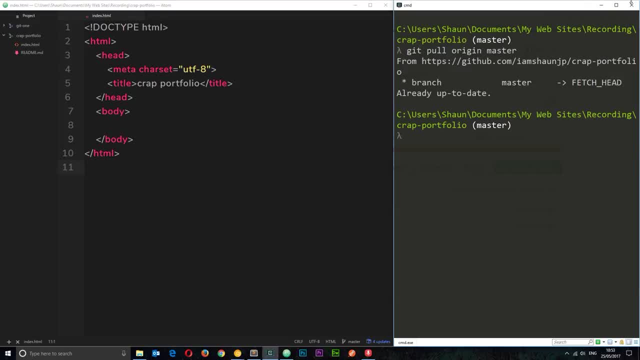 we're all up to date now. the next thing I do if I was working on a new feature is I check out a new branch, because we want to preserve the state of this master branch. we don't want to edit it and potentially mess it up. so to do that. 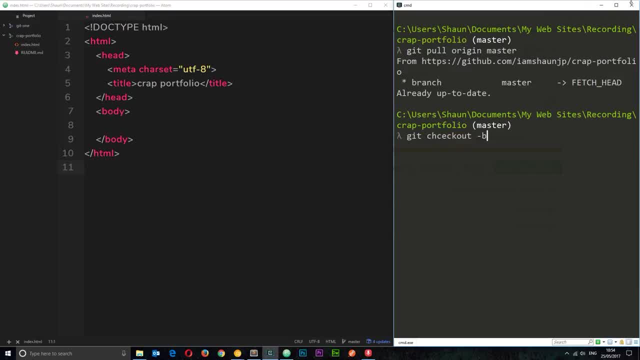 I'm going to say git checkout, then hyphen B for a new branch, and what I'll check out is a branch called index HTML. all right, because I'm going to work on this HTML page over here. so imagine now: oops, I've spelt check out wrong, so let's. 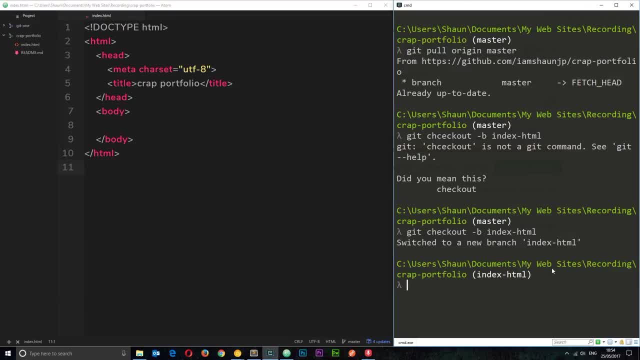 just go back and correct that. that's right cool. so on this new branch. now I'm going to go back and correct that that's right cool. so on this new branch. now I'm going to go back and correct that that's right cool. so on this new branch, now I'm 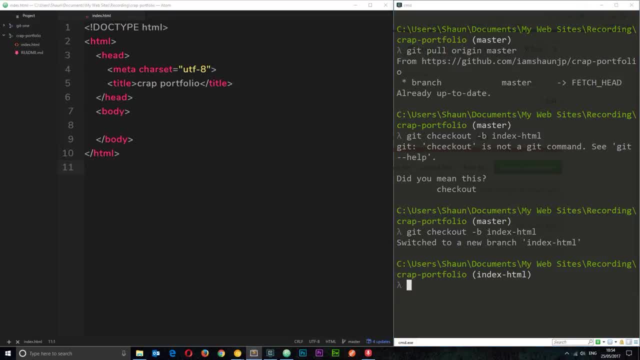 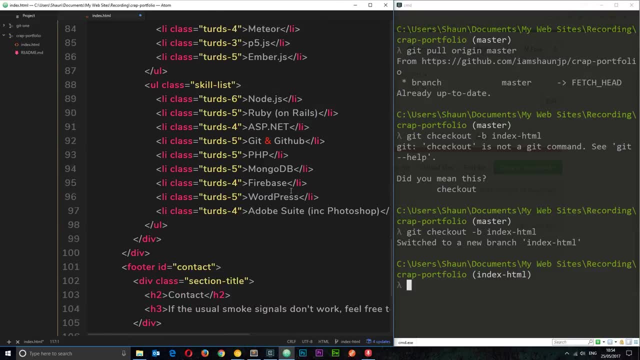 going to do is pad out this HTML file. so what I'm not going to do is just write out all of the HTML from scratch. I'm just going to paste this in right, because I'm sure you all already know HTML anyway. this is just some simple HTML to. 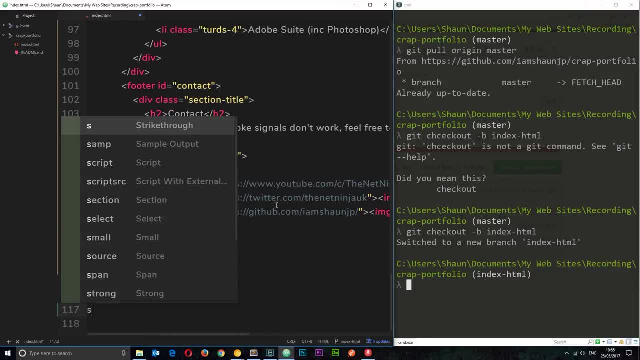 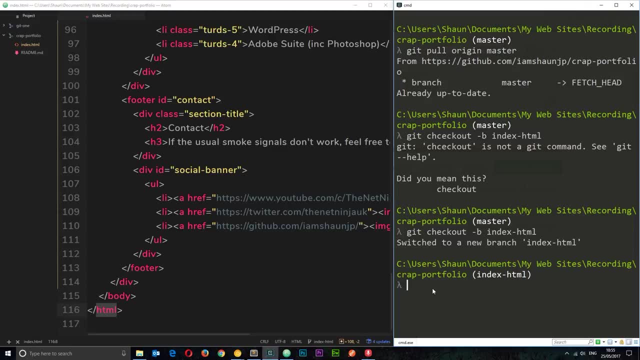 make a portfolio site. so all that's done. no, I'm gonna save it and I'm not going to add an s on the end. I'm going to save it and what I'm going to do is add this to the staging area. so I'm gonna say git add and then I'll say git commit, because 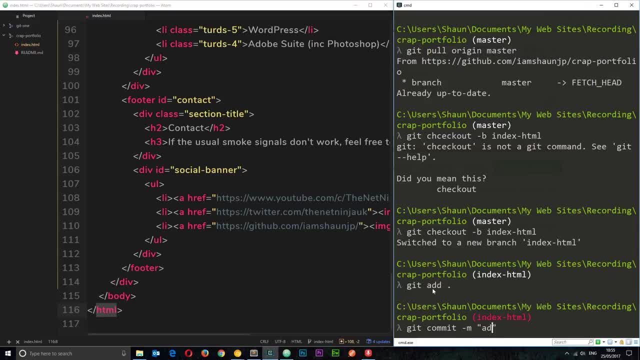 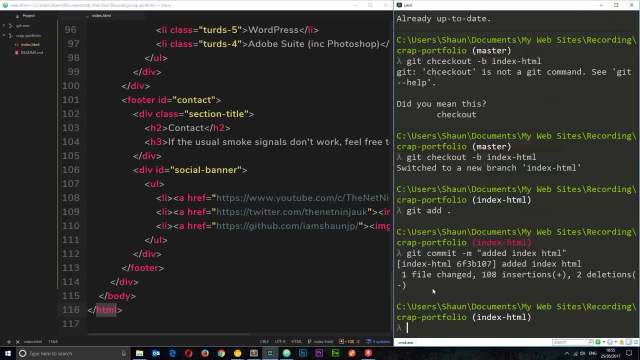 going to commit to this branch. a message is going to be added: index html. so we've made that commit and now what we want to do is take this code and we want to push it back up to the remote repository. now what we don't do, first of all, is merge this into the master branch locally and then push up. 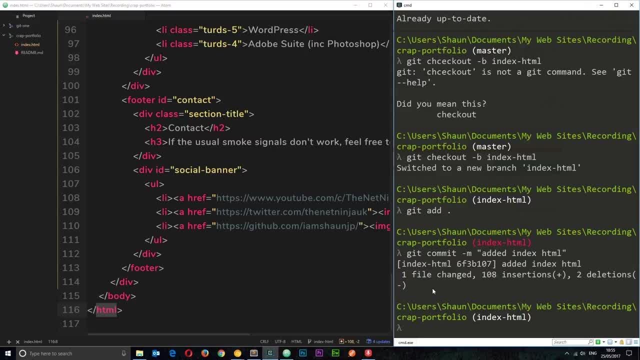 the master branch, because if we do that it's just going to override the master branch on the remote repository and the rest of my developers and my manager might not be pleased with that because they might not agree with the code that i've done. ideally, what we want to do is push this: 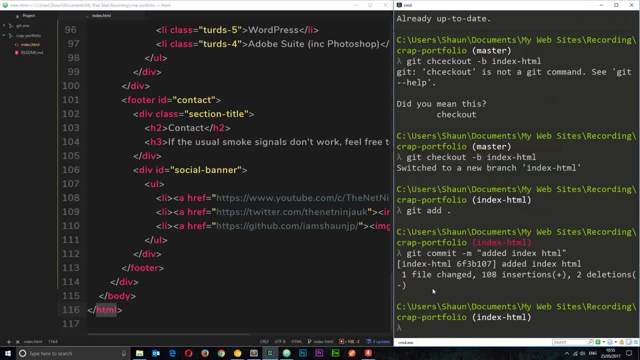 branch up to the remote so that my peers, my other colleagues and my manager can review that code and then they can all decide if we want to merge this into the master branch on the remote repository, so that everyone then can download and pull from the master branch in the remote. 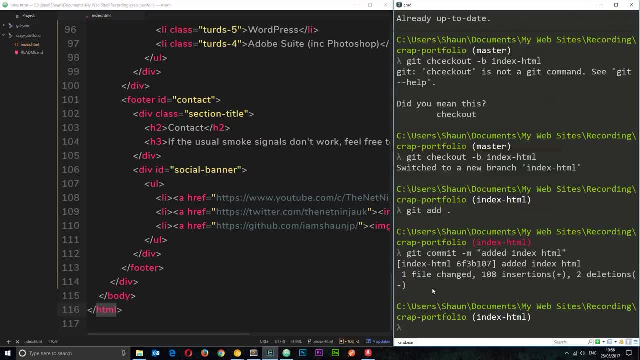 repository to update their local files make sense. so what we're going to do is push up this branch. so to do that i'm going to say git push, and then we're going to origin and then the branch name that i want to put in here is the branch name that i want to put in here, and then i'm going to 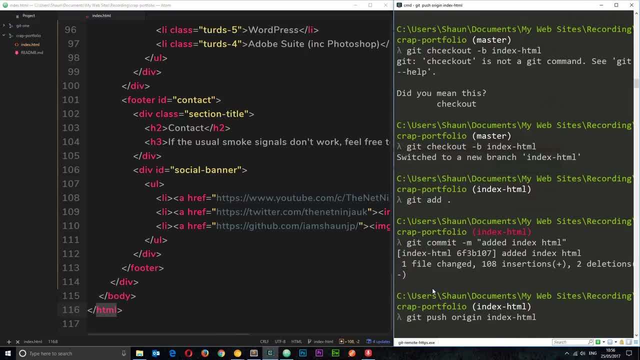 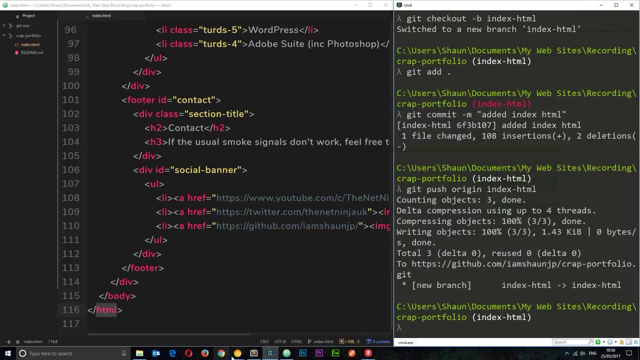 push up is index hyphen html. all right, so that is going to push up this branch and we should get feedback in a second. cool, so that's all done, and now we can check out the github repository. so you can see right here, it's auto updated already, so that's really cool. 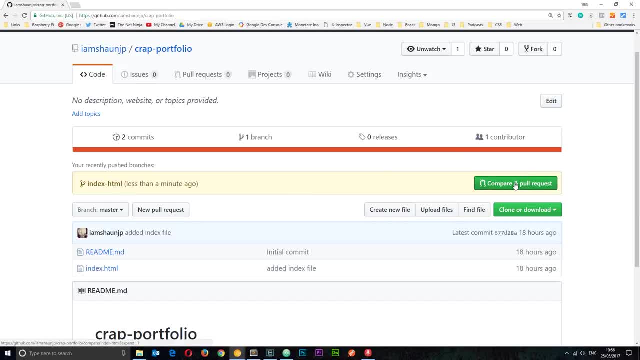 and what i'm going to do is click this button, compare and pull request, which means we're going to compare the differences between these changes and the current state of the master branch and we can then make a pull request, which means we want to merge it into the master branch. 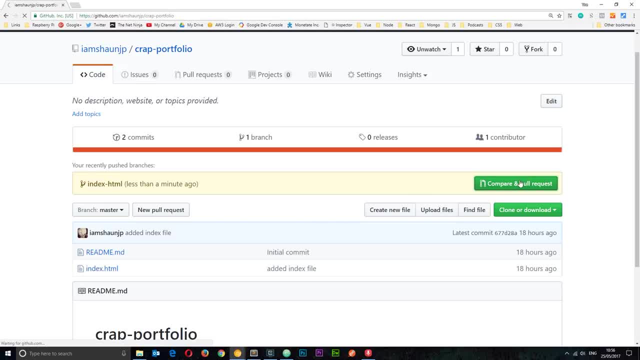 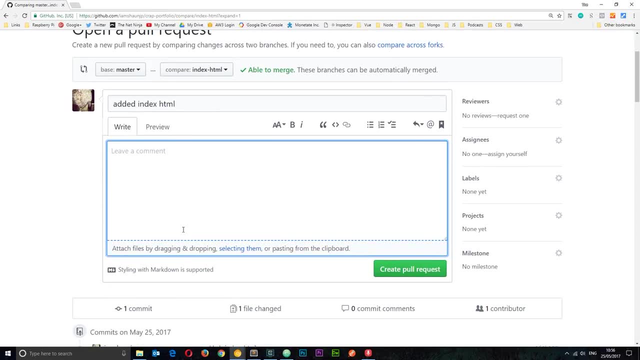 on this repository, so i'm going to do that. first of all, and on the next page, this is the message we added to the commit, which is cool. we can also leave a comment, which is good practice. you want to explain exactly what you've done, so other developers and your manager can read that, and 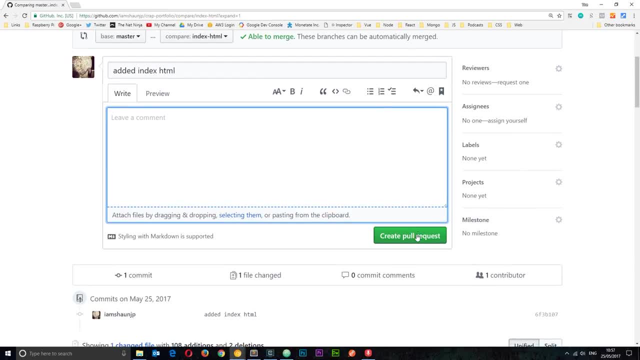 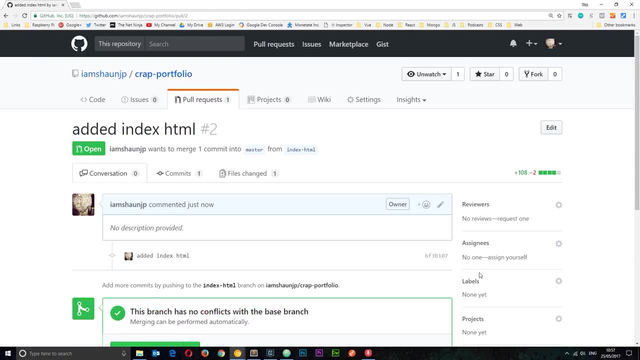 it's explicit, and then what we can do is create this pull request. so i'm going to create this pull request and that means i'm putting in a request that i want to merge this branch into the master branch on this repository right. so when i do this, other developers are going to get a lot of. 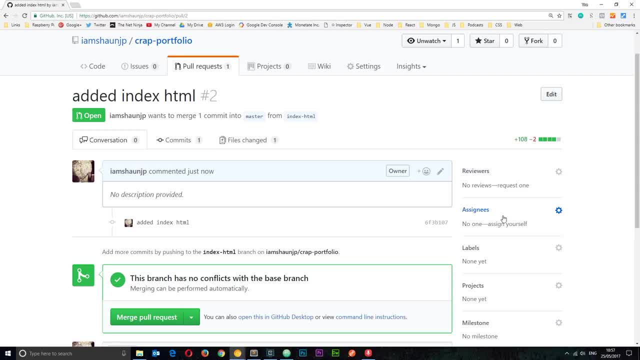 feedback and they're going to want to review this and they're going to come to this and they're going to want to review this and they're going to want to review this and they're going to get a ping or a notification and they're going to come to this and they can review it and i can assign. 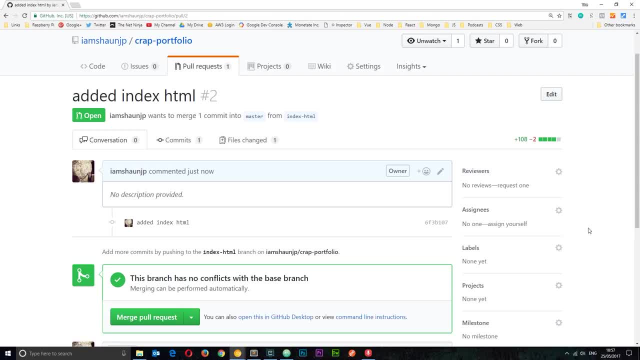 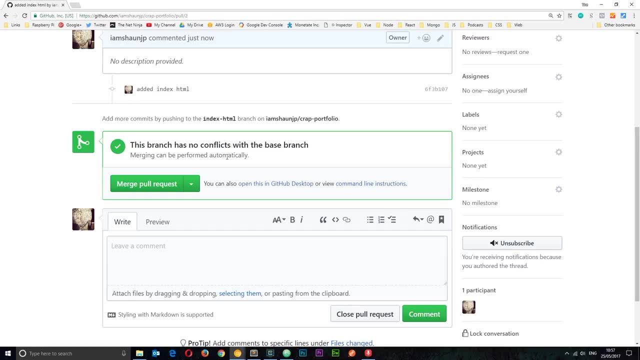 reviewers right here. currently i'm working on my own boohoo, but if you were working in a team, other people would show here and you could assign one of those to review your code so they could come down here. they could read this and it says: this branch has no conflicts with the base branch, so merging. 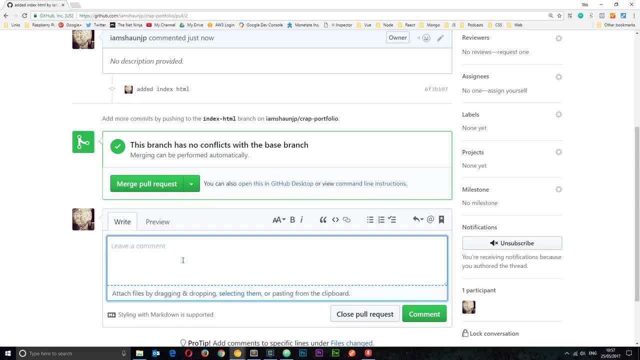 can be performed automatically. that's cool. so there's going to be no conflict if we merge into master. that's always a good sign. now, if they wanted to write a comment about this code, they they could do that here. um, i'll just put good work because it is good work. and then also what? 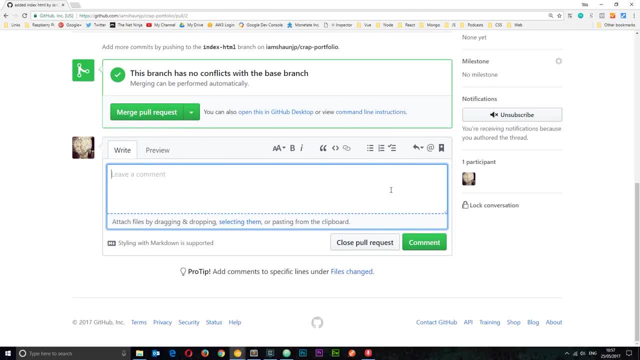 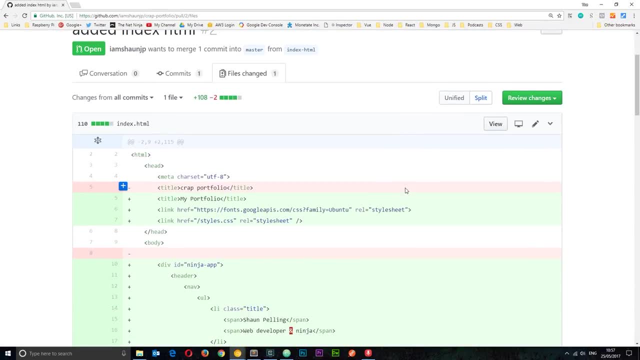 they could do is they could go down and, by the way that comment goes there, they could go down here. rather, they could go up here and they could see the commits that i've made and the files that have changed. so you can come in here and all the green stuff is stuff that i've added in. 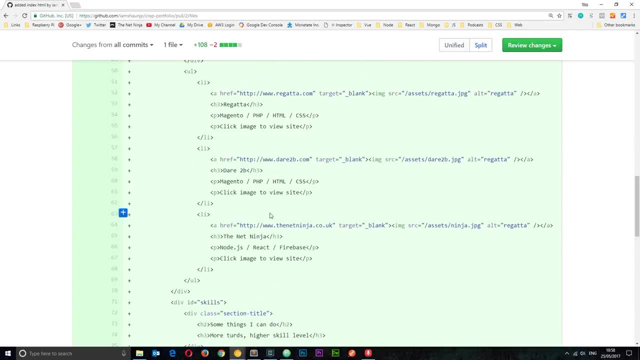 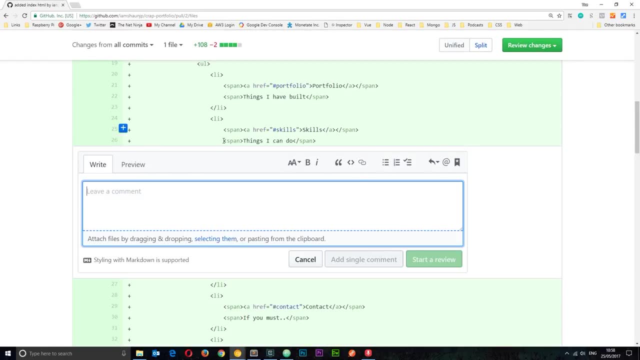 red stuff is stuff that i've deleted, so they can see all the changes in the code right there and, if you wanted to, they could add in a comment here line by line. okay, so if there's something they don't agree with, they can add in a comment there. um, i'll just put: i don't like span tags. 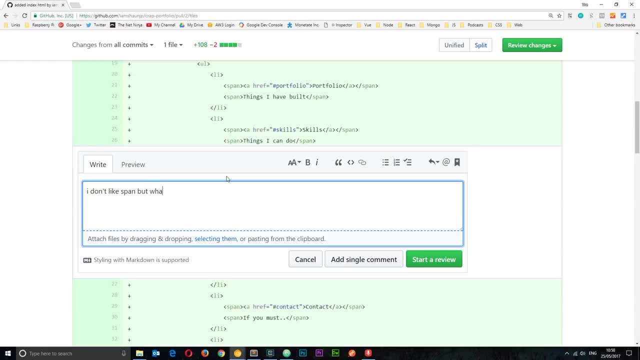 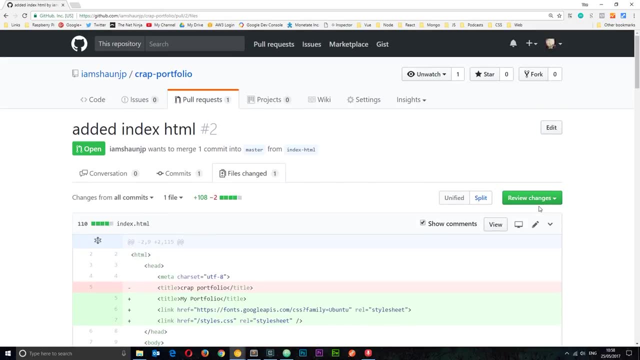 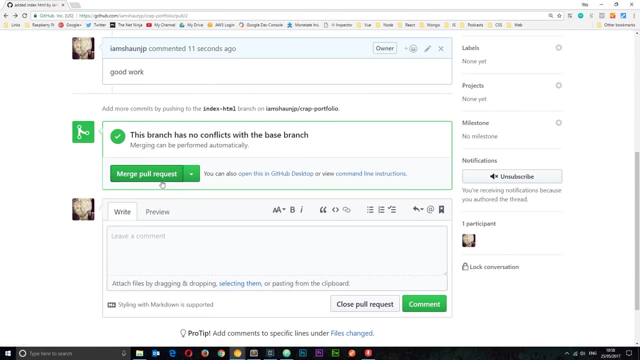 but whatevs? okay, and then we'll just add a single comment so we can do that. and then, if we're all happy with it, we can go back to the master, to the- uh, the request, sorry, and we can merge this pull request right. so if we merge it and confirm merge, what that's going to do is take this branch. 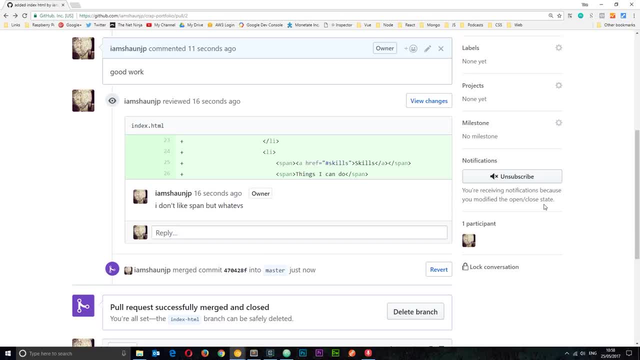 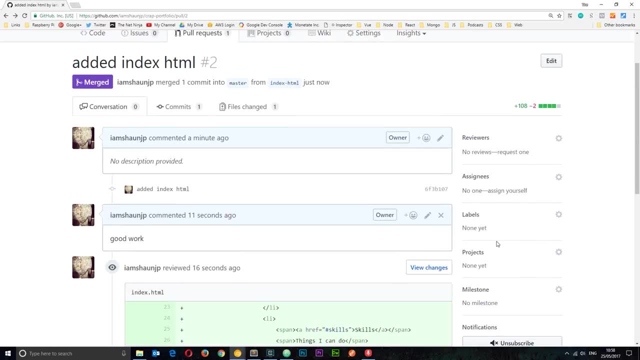 that i've uploaded and it's going to pull it up. and it's going to pull it up, and it's going to pull it, or rather merge it into the master branch right. so now, if we wanted to, we can delete the branch as well, because it's already been merged. and then, if we go now to crap portfolio to see: 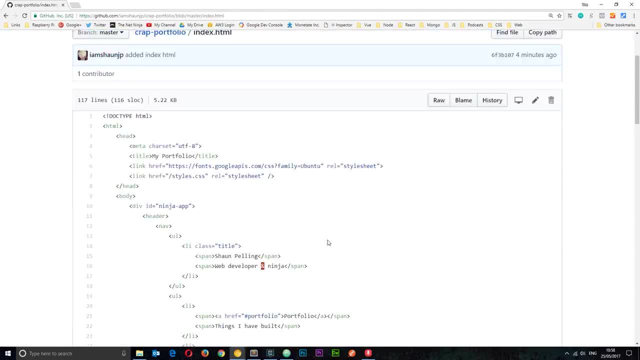 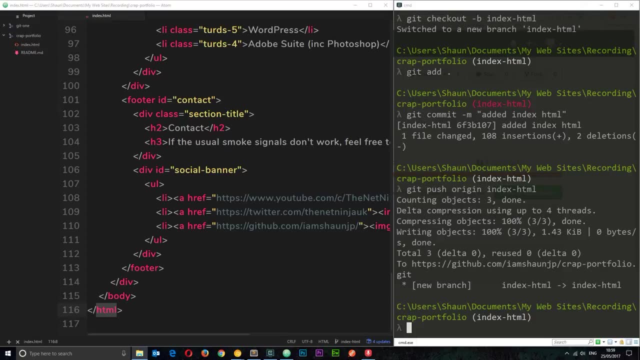 the code. we're going to see this index. this is the master branch we're on updated. so now we've updated the master branch, cool, right, okay. so imagine, a few hours later someone's been onto the code and they've seen that i've missed out the images and they say, hey, you need to put these. 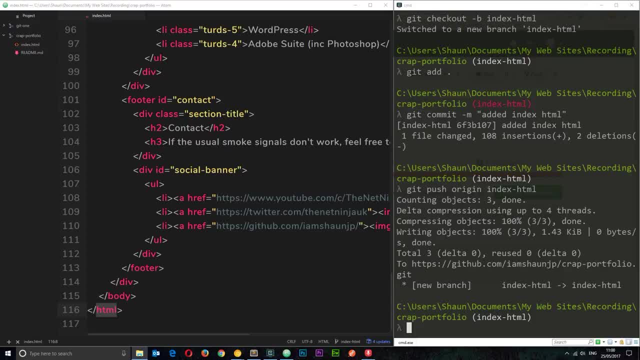 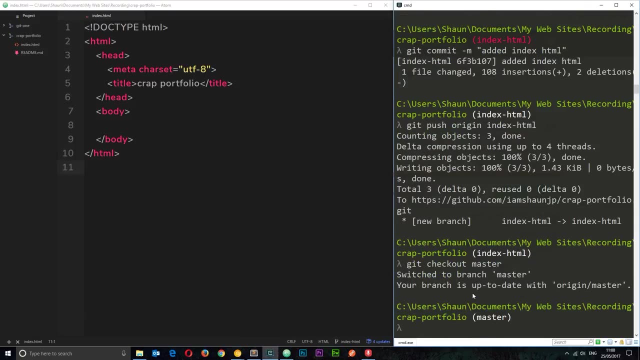 images in. can you re-upload this? so i say okay. well, whatever, what i'm going to do is start a new feature. i always need to pull down the master branch just in case anyone's made any changes. so what i'm going to do is go to git checkout master to check out the master branch and then 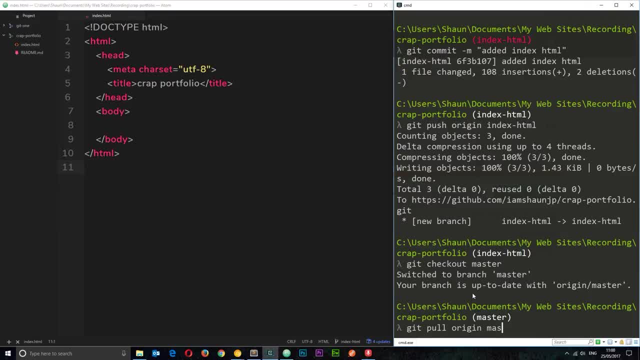 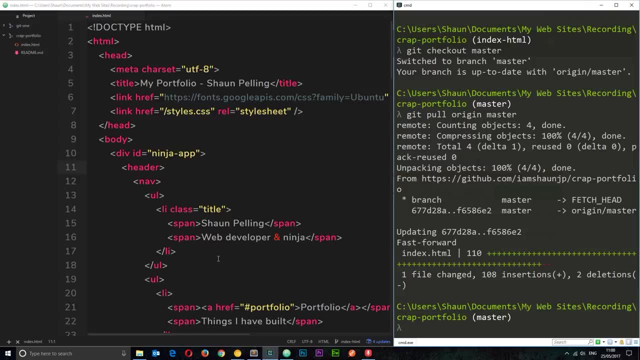 what i'm going to do is say: git, pull origin master. okay, now this time it is going to pull something down and you can see we've got changes now. so it's updated the index page and someone's made a change as well. so the change i made in the last section where i uploaded that branch. 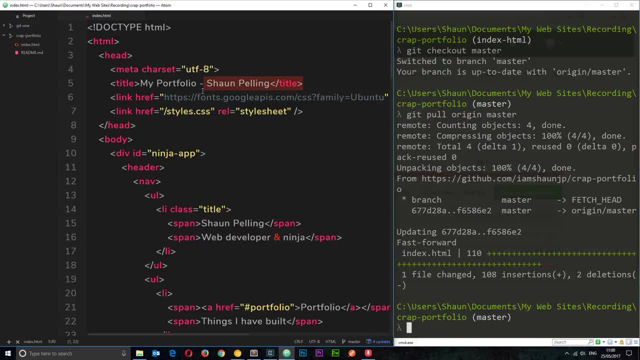 has come down and also someone else has made a change to this title as well, so we've updated that. it's always good practice to update the master branch first of all, to pull down, and then what we're going to do is check out a new branch for this new image feature. so let's say, git checkout. 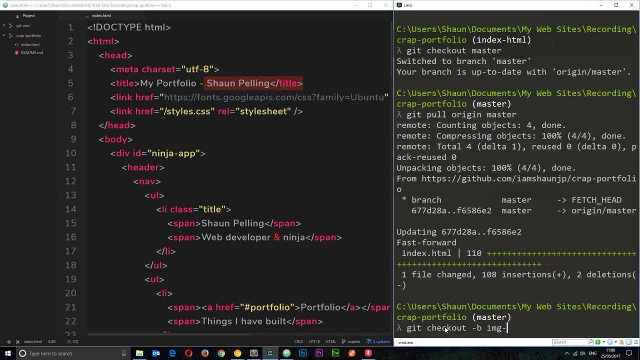 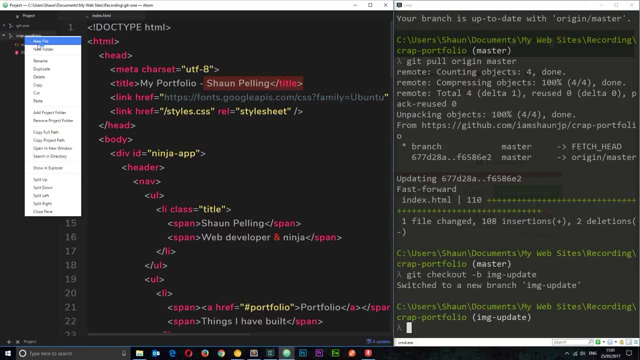 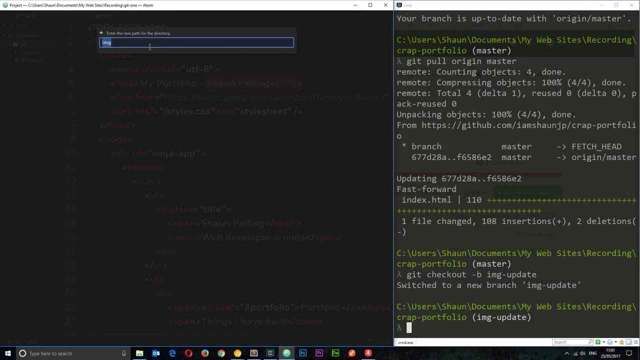 and then hyphen b to say new branch, and then image update. okay, so now what we're going to do is we're going to add in the images, so we'll right click over here and we'll go to new folder and i'm going to drag. in fact, we'll rename this, let's call it assets, okay, and then what we're going to do is: 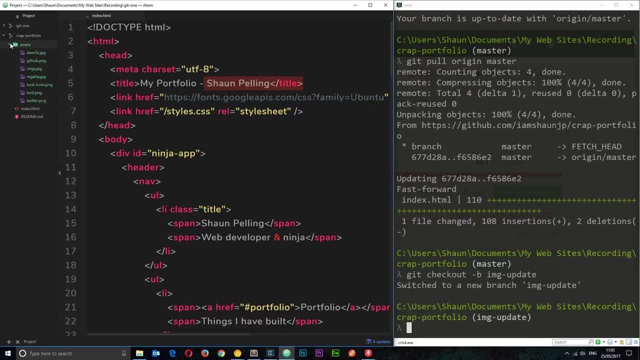 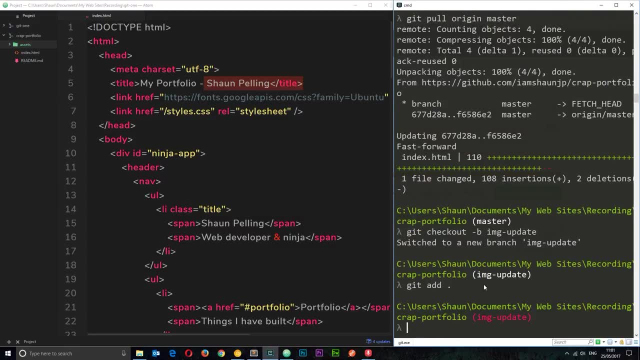 just drag these images in now. i've already made these images and now you can see all of these things right here. okay, so now what we can do is we can say git add, that's going to add everything. then we can say git commit m. then the message added images and you can see all those have been. 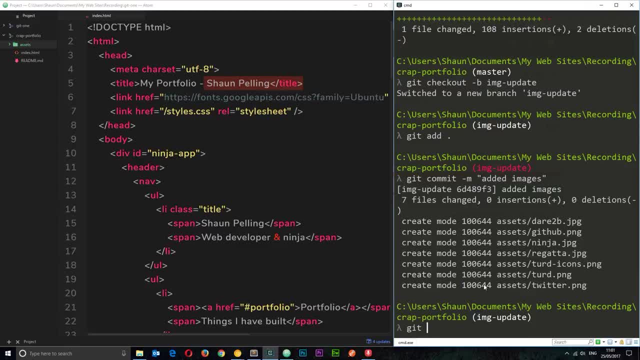 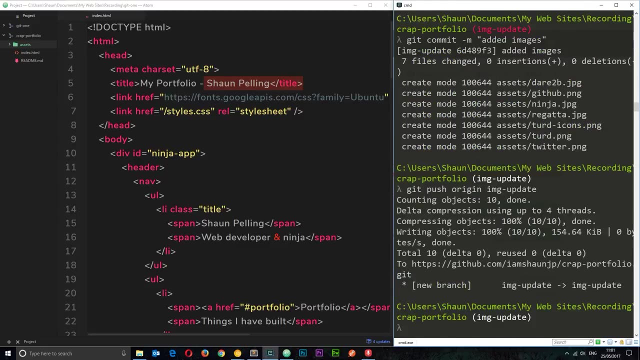 updated there. now what we're going to do is push this image in and we're going to go to the remote repository. so i'll say git, push, origin, and then the branch name was image update. so amg update, click, enter. cool, so that's now all done. so i can check out the remote repo and if we come over here, 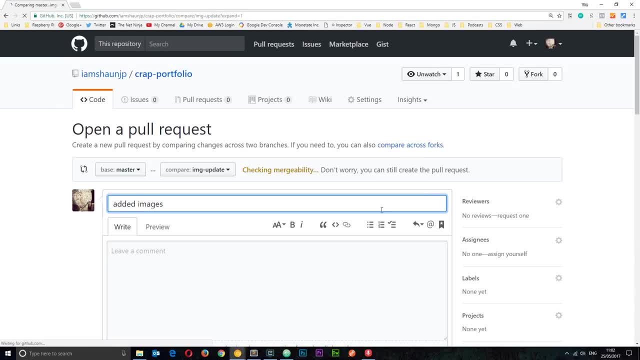 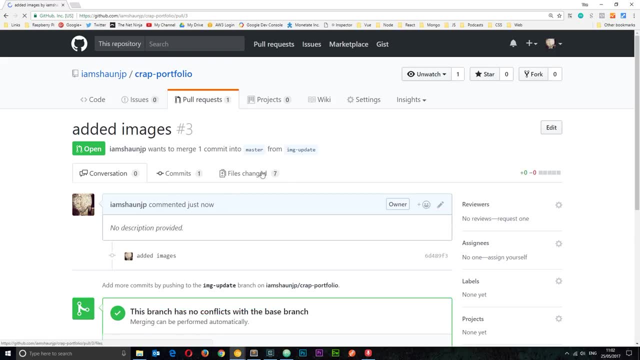 we can see that branch. so again, i'll compare and pull and you can write a comment in here if you want to. um, what i'm going to do is create this pull request and then we can see the file is changed over here. if i was a reviewer or the manager, i could come over here. see all these. 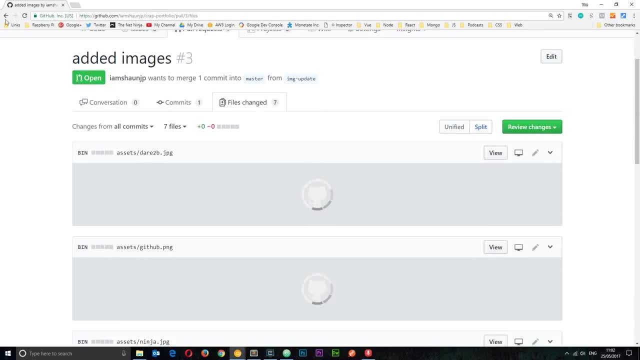 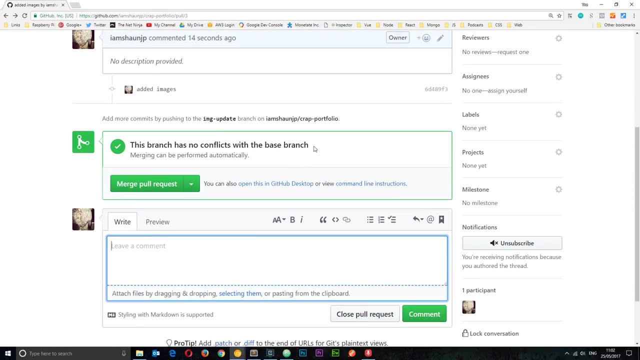 different images that have been uploaded. i'm not going to wait for those to load, because my internet is really bad at the minute for some reason. anyway, go back. so those files have been added. so i noticed that one's missing. so i can say, hey, can you add the missing image, all right? 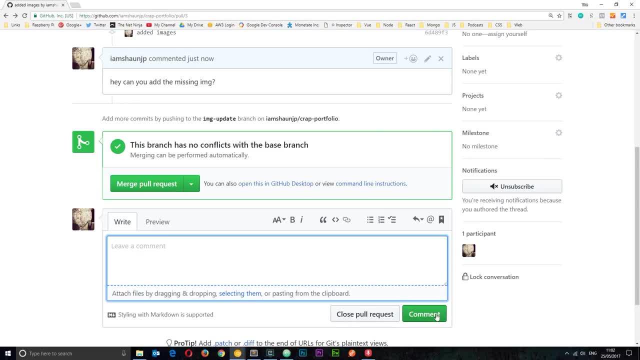 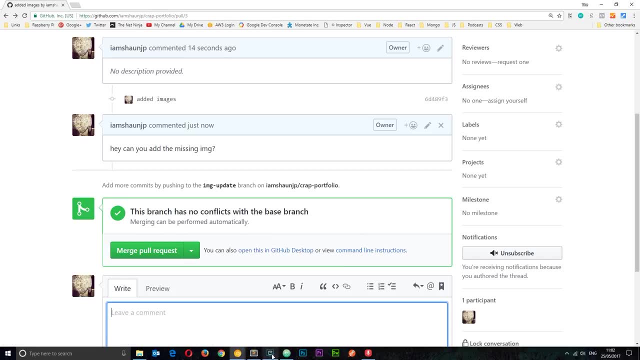 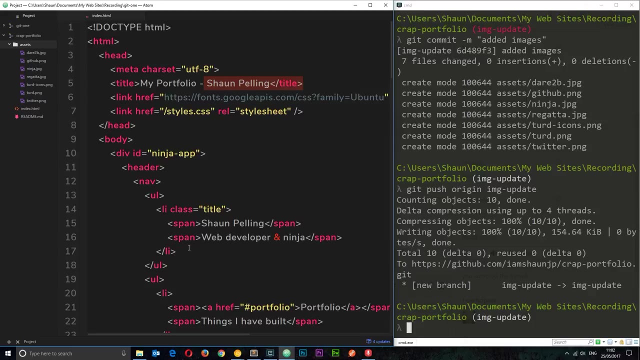 so i'll comment that there. so i want this person to add the missing image before we merge this. okay, so what i do is i go back to my code and i notice i have in fact missed an image out down here. so i don't need to switch branches. i'm going to stay on the same branch because we've not merged. 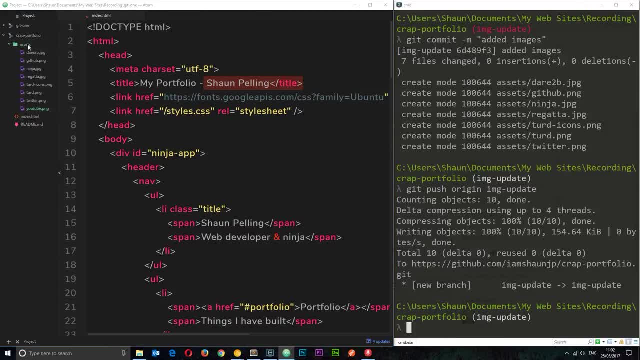 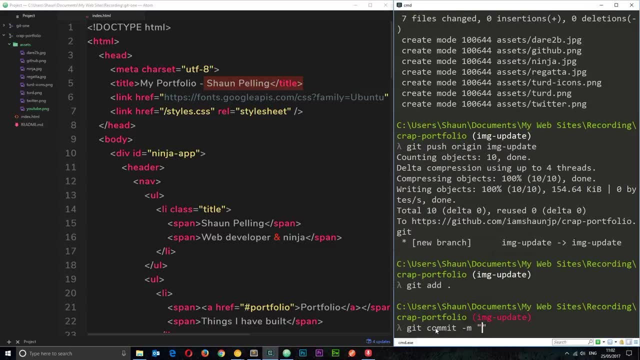 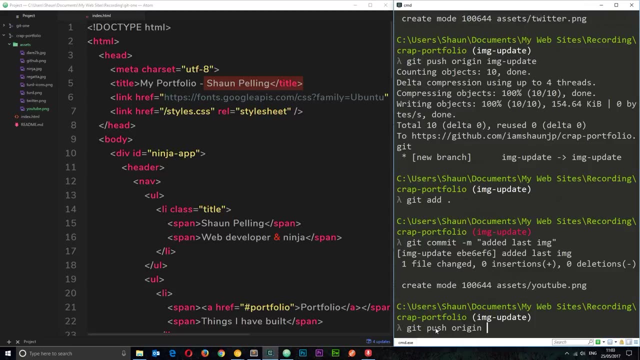 it or anything. yet what i'm going to do is drag in the last image that i missed, and then what i'll do is say git add, and then i'll say git commit, um, and the message is going to be added- last image. then i'll do a git push again. i'm going to origin and still the same branch, because we're still on. 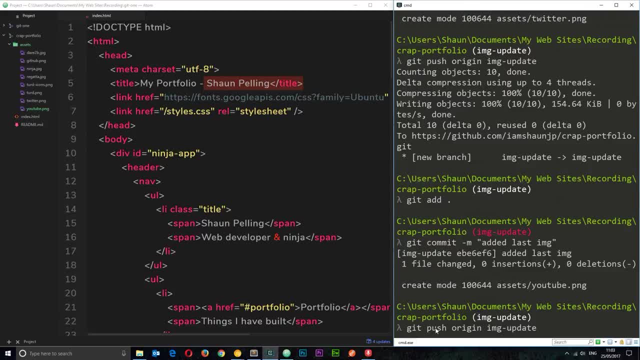 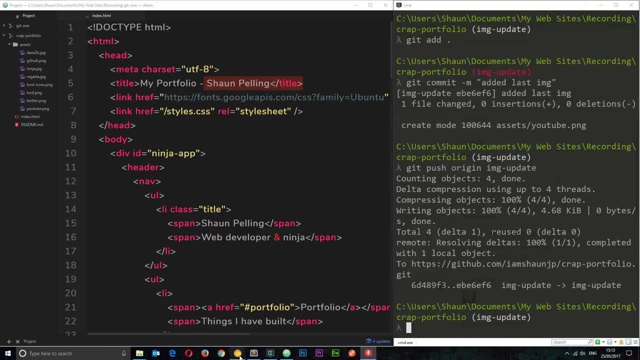 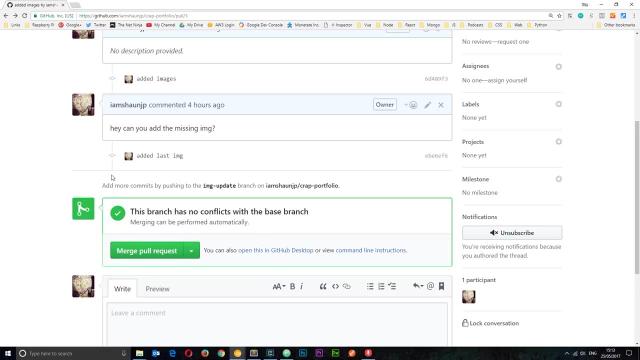 the same branch, so we're just pushing a further commit basically to this same branch on github. all right, so now that commit's been pushed up to github i can go and check out the remote repository and we can see right here: added last image so that new commit has appeared on this timeline down here. 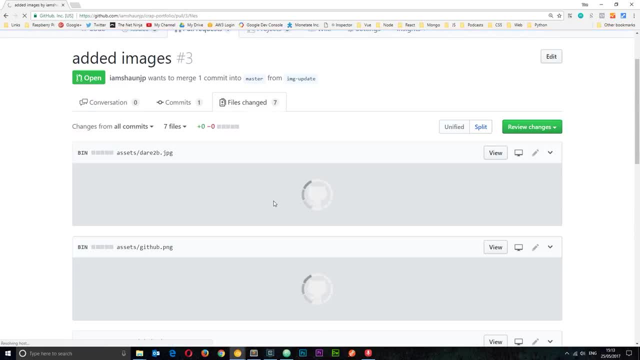 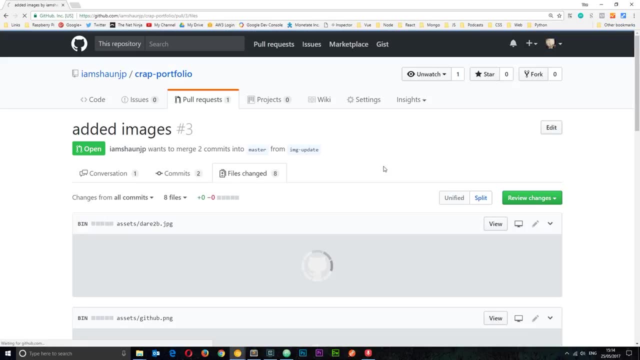 so i can just view that over here if i wanted to. and it says this page is out of date. refresh because there's now an extra file changed. so now it says eight files changed and now it's now we can see all of those files down here. so as the manager now i'm completely happy with this and 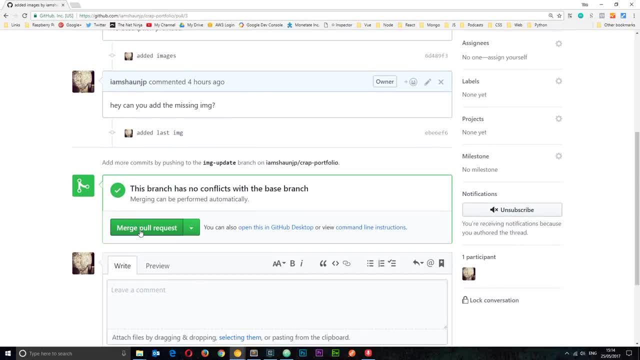 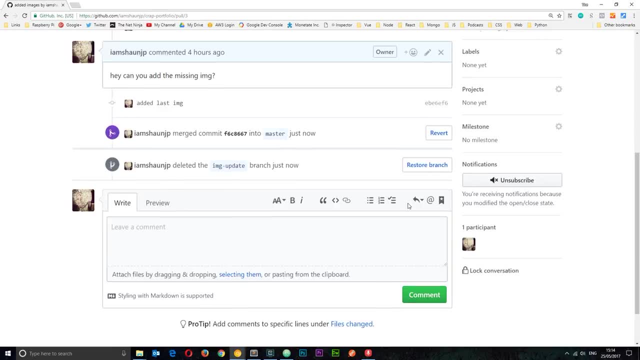 i'm happy to merge this into the master branch. so i'm going to merge this pull request, which is going to take all of these images and add them into the master branch. i can delete the branch if i wanted to. um, you don't have to delete the branch, by the way. um, you can keep it so you can refer to it in. 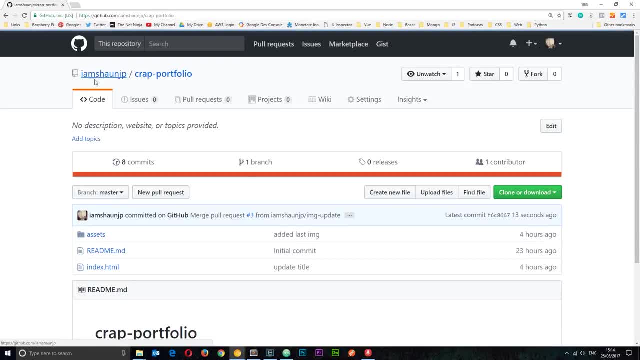 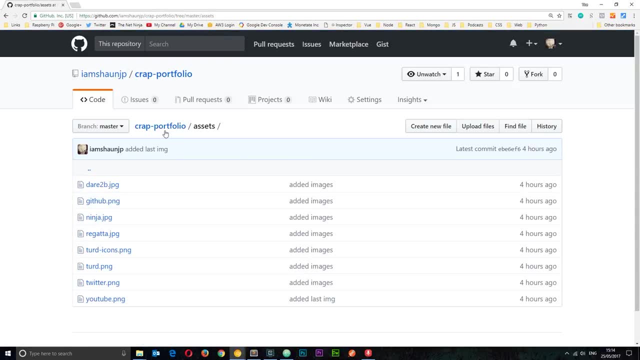 the future, but i'm going to delete it in this case. so if we go to the code now, you can see what on the master branch and we can see now this assets folder and we can see that we've added all of the images and we can see that we've added all of the images inside it. okay, so that's how i typically do. 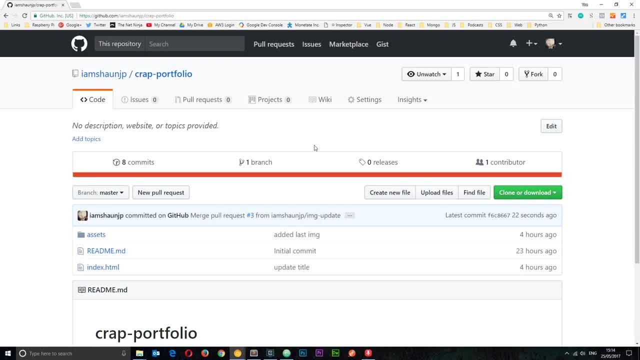 things on github if i was working on a project with different colleagues, because then, as i'm pushing up these branches and merging the branches, what my other colleagues would be doing is pulling down from the master branch. so any updates that i've done emerged, they're going to get in their